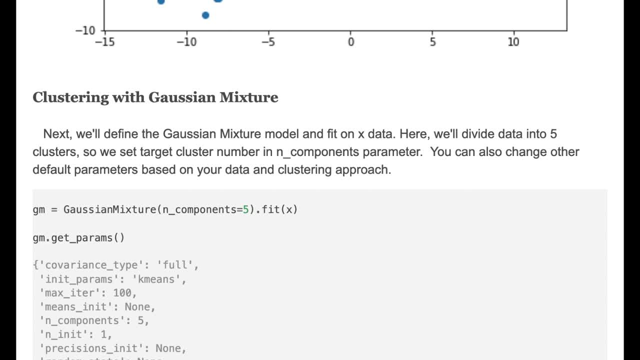 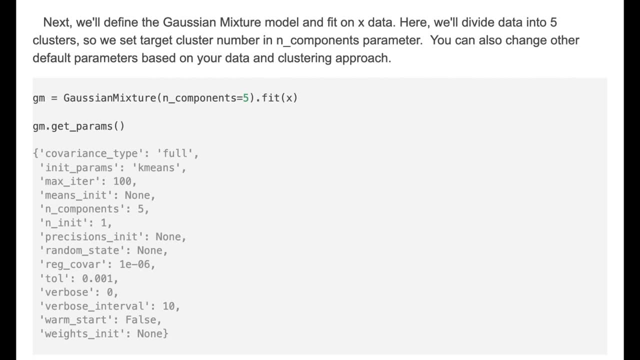 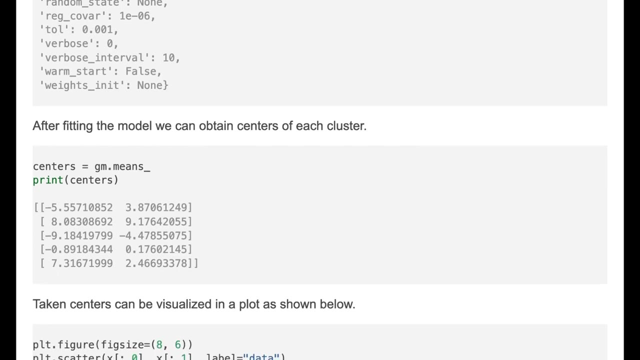 You can also change other default parameters based on your data and clustering approach. Here is the source code, how to define the model, And we'll you can see the parameters used in this model. After fitting the model, we can obtain centers of each cluster. so we have five centers. 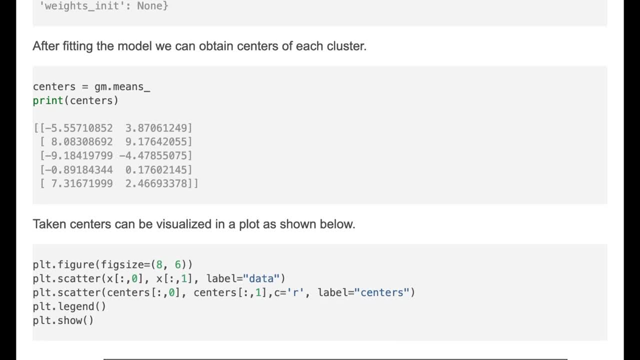 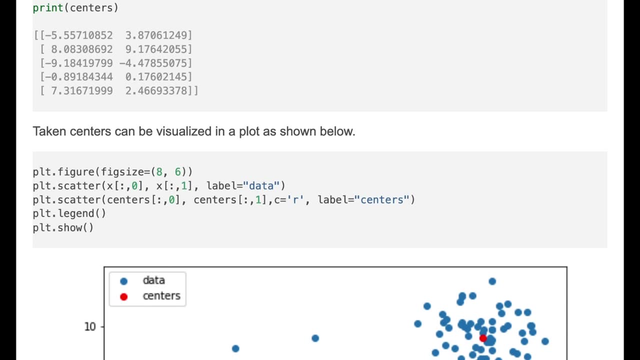 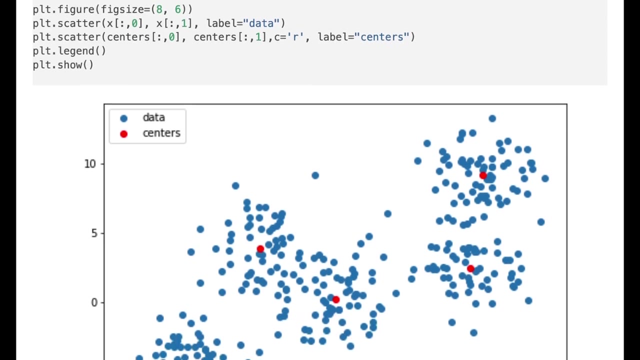 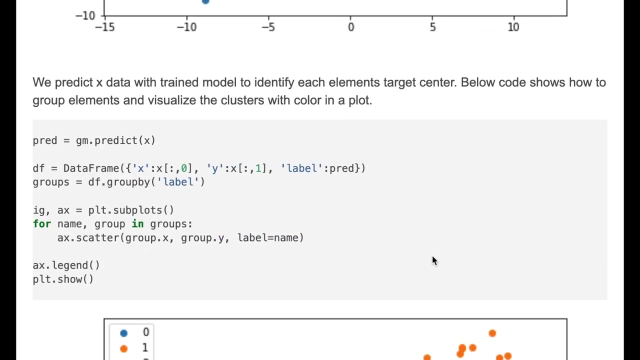 so this is the values of the center Taken. centers can be visualized in a plot as shown below. so again, we visualize the scatter plot and highlight the centers of each cluster with a red color. So we found five clusters in this plot. 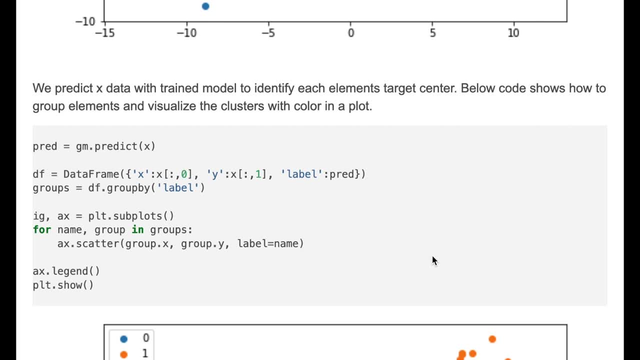 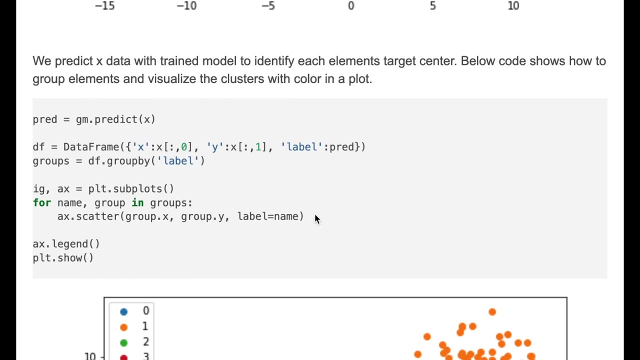 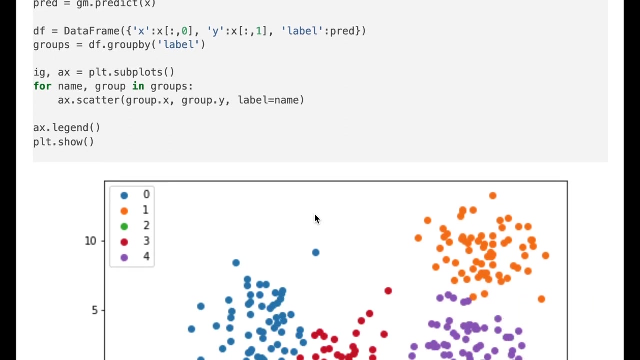 We predict X data with trained model to identify each element's target center. Below code shows how to group elements and visualize the cluster with color in a plot. Here we use data frame and group each cluster and we highlight each, every cluster, with a color. 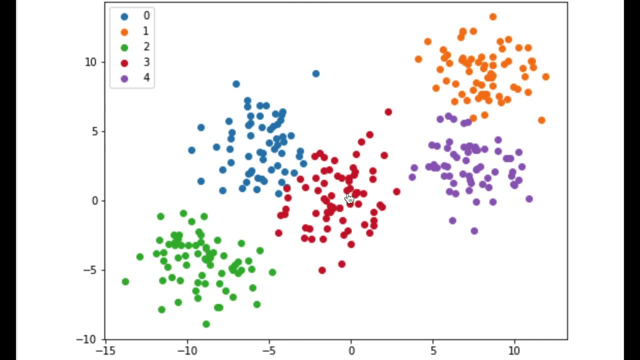 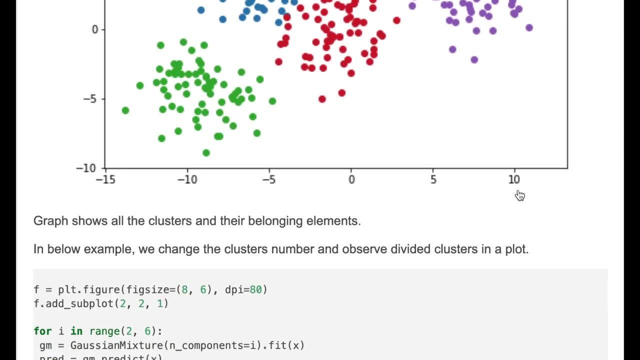 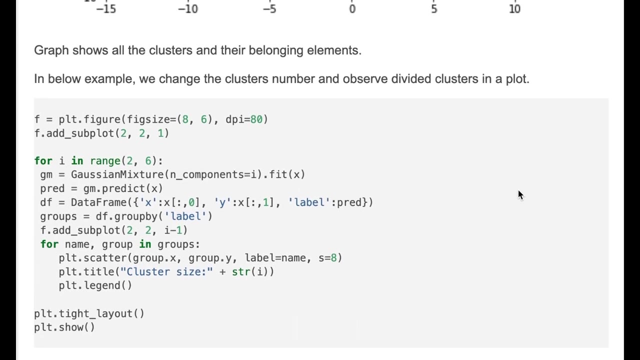 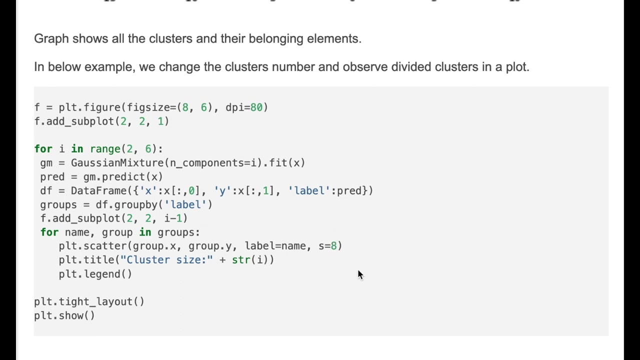 And this is the result. Here we have the five clusters highlighted by different colors. In below code we change the cluster number and observe divided clusters in a plot, So you can test your data by changing the cluster numbers. This is the source code: how to identify the clusters. 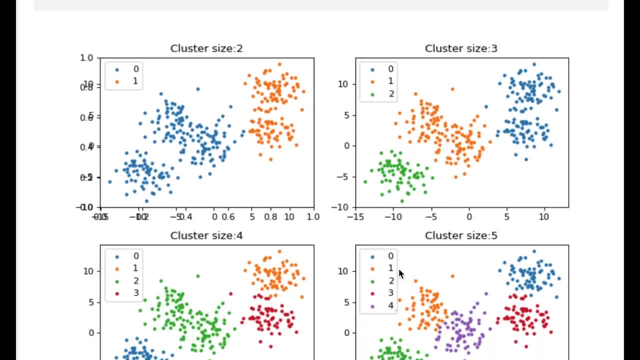 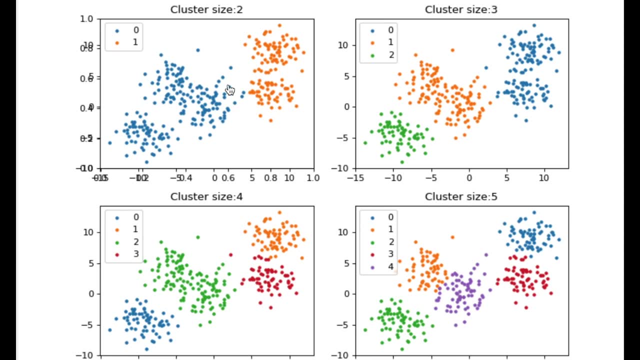 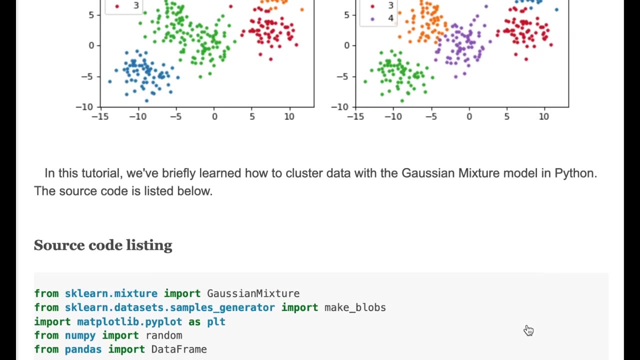 And check And here we have the output result. So this graph shows: in the first graph we divided into two clusters, So cluster size is two And the second one is we have three clusters and four and five. In this tutorial we have learned how to cluster data with the Gaussian mixture model in Python. 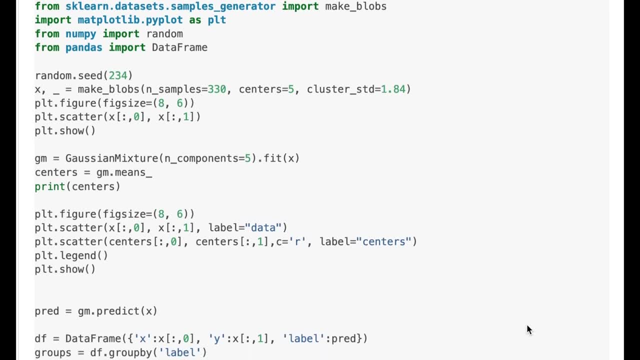 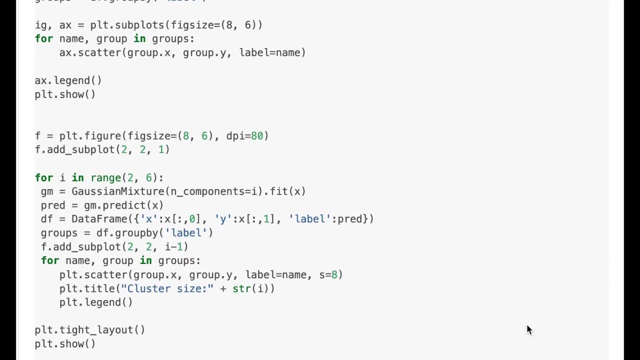 And here is the source code. Please visit my website. You can get all the source code And all the information we have covered here. Please subscribe my channel and hit like button if you like this video, And thank you for watching and see you next time.